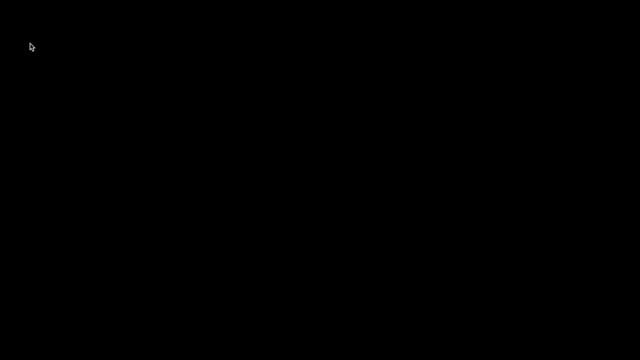 Hey, let's talk about multiplying variables. So when we're multiplying variables generally, you'll see something like this: 4 multiplied by x, And a lot of people get confused when they see the 4 and the x right next to each other. 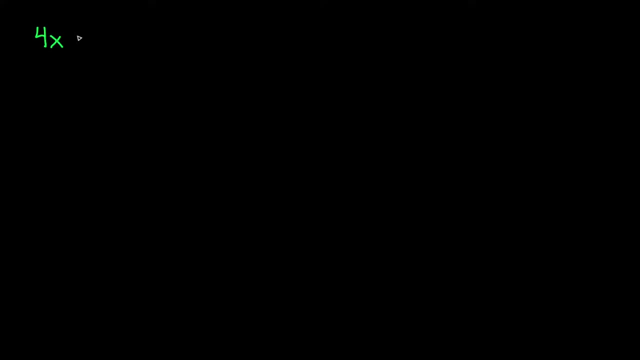 And you know understanding that that's multiplication And they wonder why we don't do something like this. But once you write it out it does become a little more obvious. you know why we won't do that And it's because it gets confusing. So imagine we were writing 4 times x. 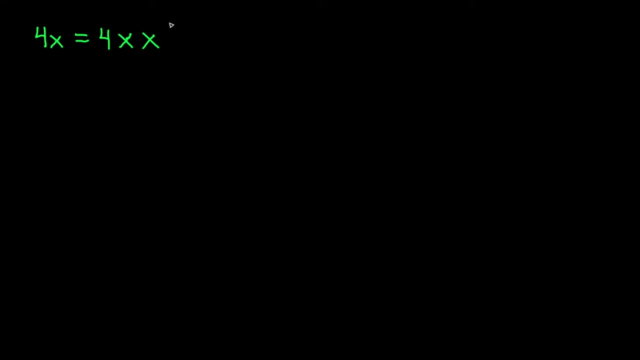 Now we just have 4xx And it looks kind of confusing, It looks unorganized. It's a little harder to tell. you know that 4 is associated with this x over here, So that's why we write the 4x like that, Or sometimes it's 4y. 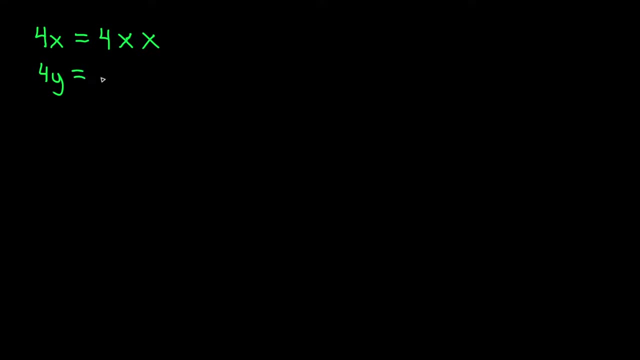 It just it looks more organized. And 4 times y would be equal to 4.. Well, 4y would be equal to 4 times y. So let's say we're told that y equals 2.. How would we do that with 4y if we were given this? 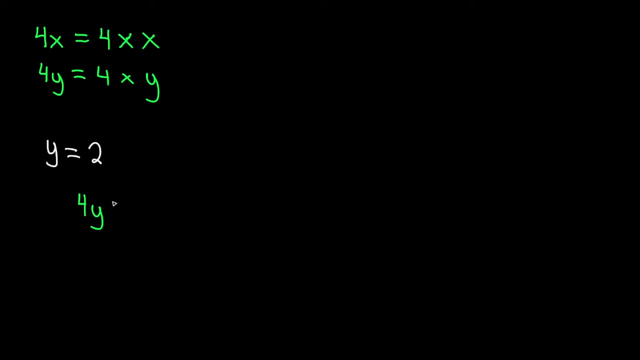 4y. Well, 4y 4y, we already know, is equal to 4 times y. So we could plug it in like this: 4 multiplied by 2.. Or you could just look at it like this: 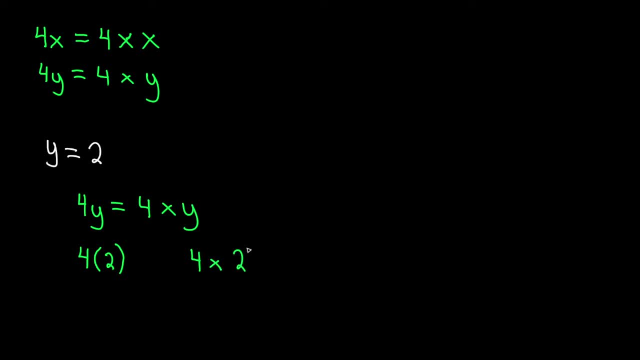 4 multiplied by 2. This comes out to 8.. This comes out to 8.. They're the same thing Generally. Generally, though, you will see it like this with the parentheses. Like you'll just find it easier to put it into parentheses, where you have your variable. 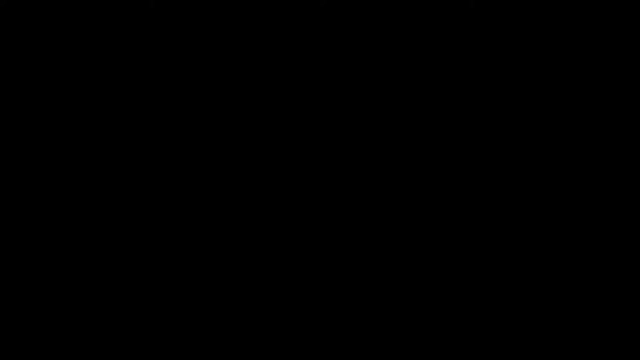 Let's scroll down here. I'll do a few examples. Doing examples definitely clears things up more. Say, we have 4x And we're told that x is 3.. So what we're going to do is just say, all right, x is 3..